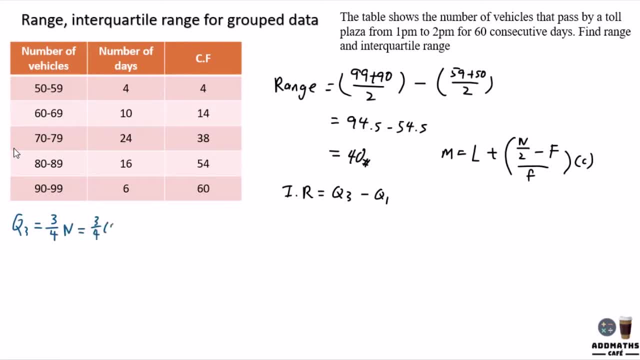 so 304 of your m means 304 times 60, it will give you a 45. and for q1 it will be 104 times n, which means 104 times 60, which will give you a 15.. so let's look at the cumulative. 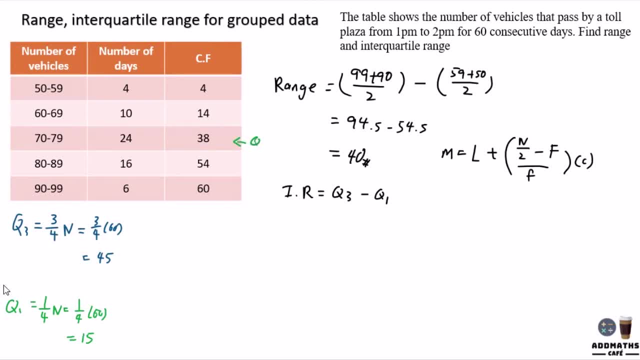 frequency. your q1 will be at this part, as 15 is in the 38th, and for your q3 it will be in this part, as 45 is in your 54. so focus in this two group. first, to find q3, simply apply the formula. so q3- the lower body over here- is 79.5. 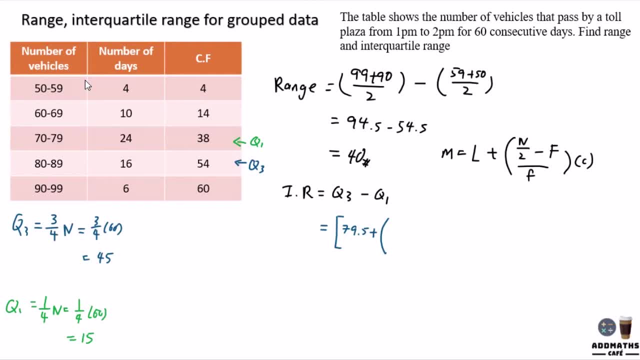 plus your n over 2. now change to your 304n, which is 45, minus your big f. big f is your cumulative frequency of previous data of this previous class, which is 38, minus the frequency of the q3, which is 16 times the class, which is 10, and then minus your q1. so say, open a big bracket, your q1 lower body is 69.5. 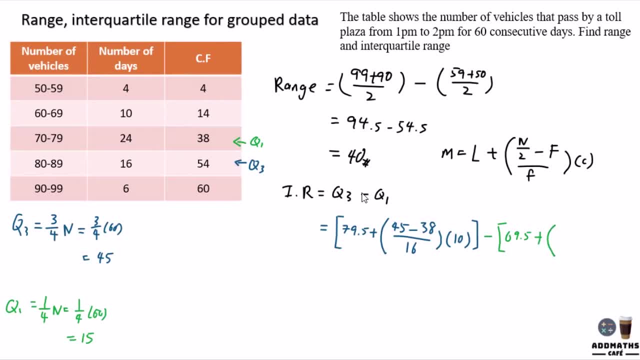 plus. now your median is n over 2, but your q1 is 1 over 4n, which is 15.. so apply 15 minus the cumulative frequency of previous class, which is 14. divide the cumulative frequency of your class, this q1, which is 24 times the class. 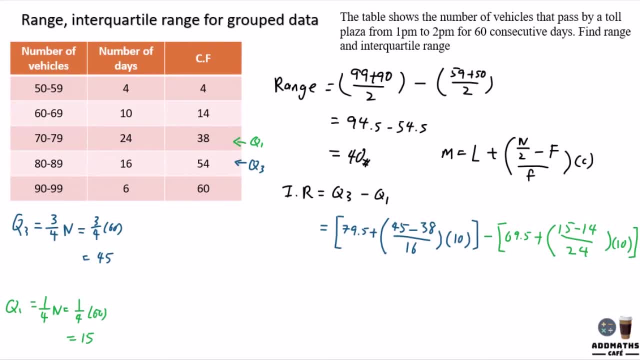 okay, in this case you have to get your calculator to do the work and in this part it will be 83.875 minus 69.987. so in this case your interquartile range will be 13.958.